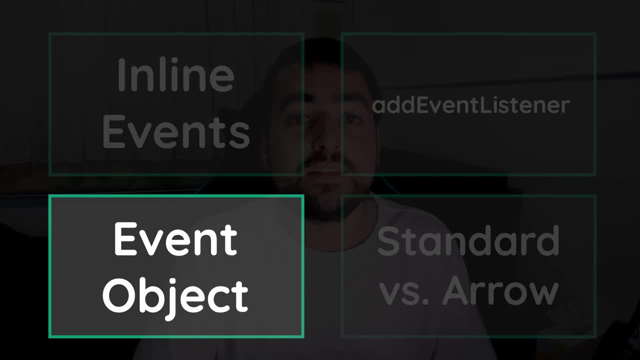 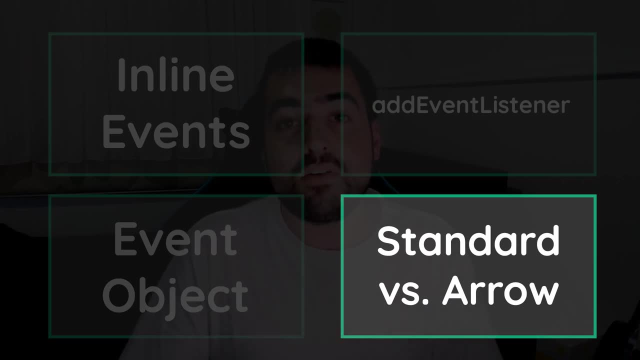 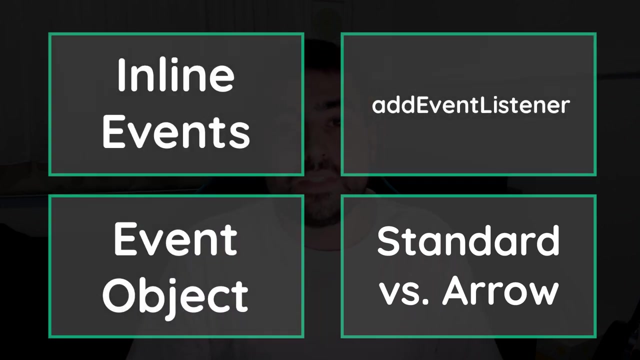 right here are going to tell you information about the event which just occurred, And the last topic is going to be the difference between a standard JavaScript function and an arrow function when it comes to the events. So hope you guys enjoy and learn something from today's video. Let's get right into the first topic here, the inline HTML events. Okay, 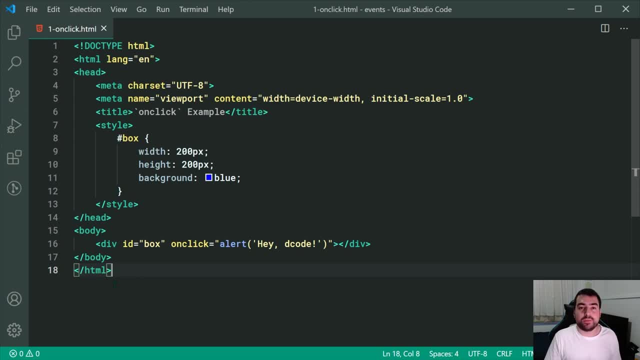 so, starting off with the most basic form of a JavaScript event handler, Okay, so right. So right. here I've got a fairly straightforward HTML file and we can see right down here. I've got this div with an ID of box and I've applied some fairly straightforward CSS styles to 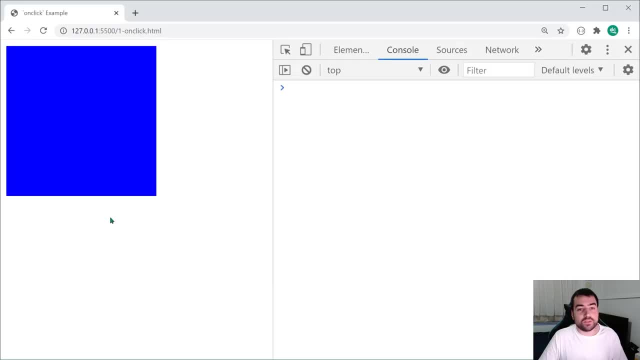 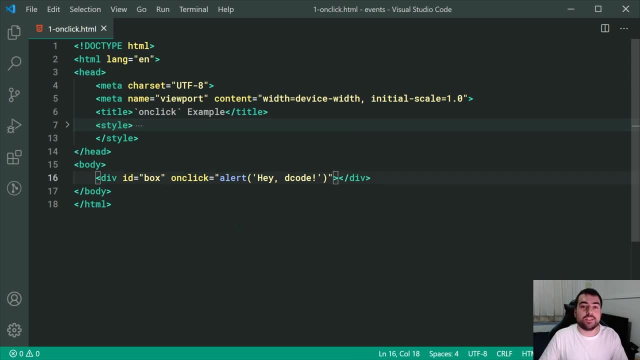 this box. So now we can see in the browser it's going to look something like this. So if I go back inside the text editor we can see inside the actual HTML for the box itself. we can see it says onClickAlertHeyDecode. So this right here is the most basic form of a JavaScript event, and you'll find this. 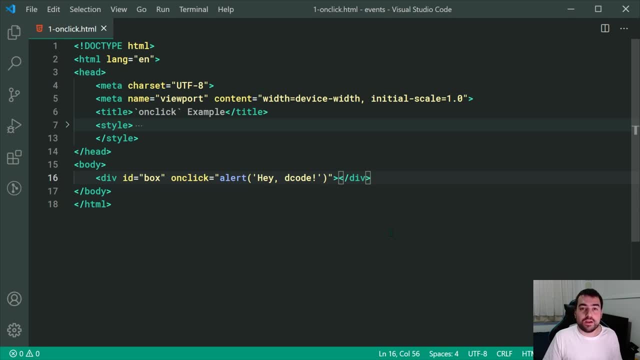 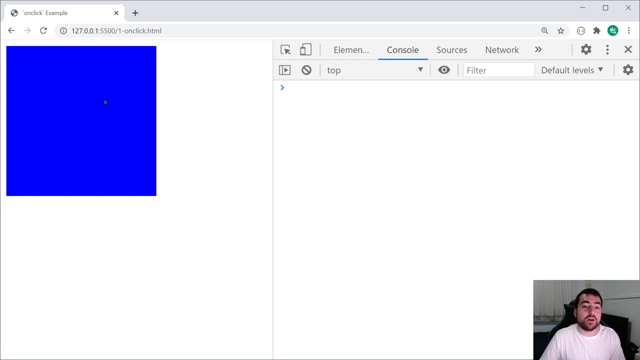 style on many different beginner tutorials out there on the web. Now, of course, it's quite self-explanatory what this does. When I click on the box, I want this to say: AlertHeyDecode. So now, if I was to go inside the browser, we can see upon clicking on the box. we, of course 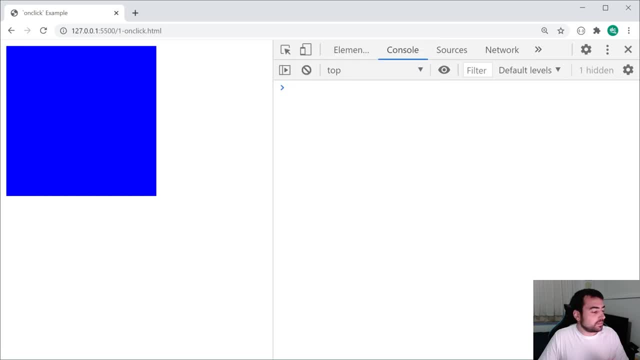 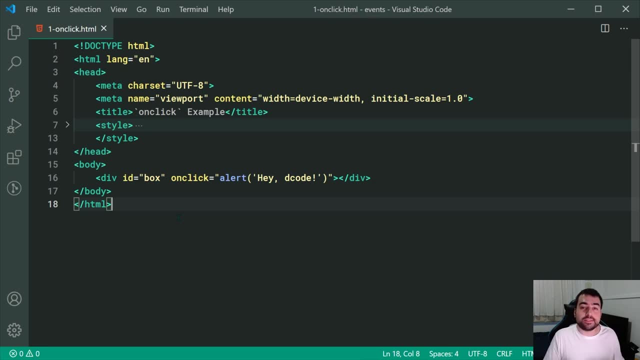 get HeyDecode right there, And that is the most basic form, like I said, of a JavaScript event. Now, of course, if you're using a text editor like Visual Studio Code, if you go inside the actual div here and you specify, for example, on or just on, we can see there are many different. 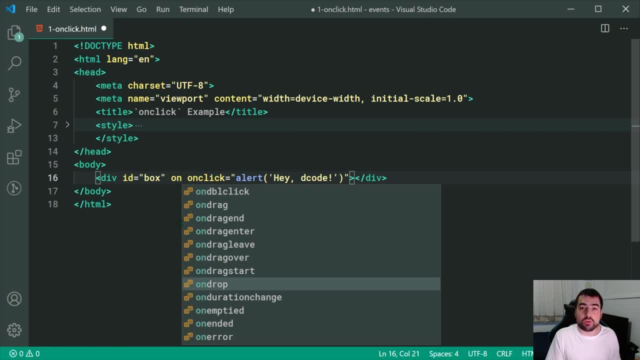 events to choose from And, of course, when doing your own project, you're going to be googling these things and finding out exactly what type of event you need to use for your own scenarios. An example might be the onMouseOverhead, And essentially it's going to allow you to react to when the user hovers their mouse. 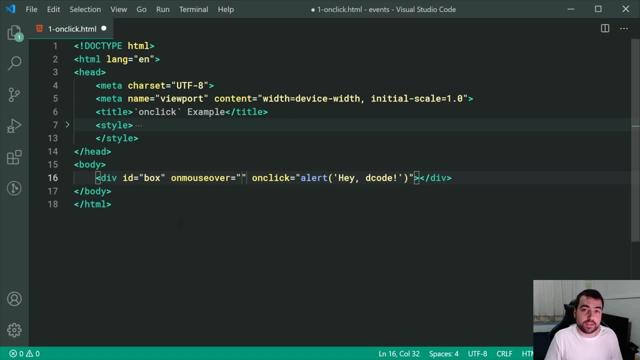 over the actual div or the box, in this case right here. So for example, I can just say Alert, then I can say something like Hover, Just like that. So now, if I was to save this, we can see. of course we actually have two event handles. 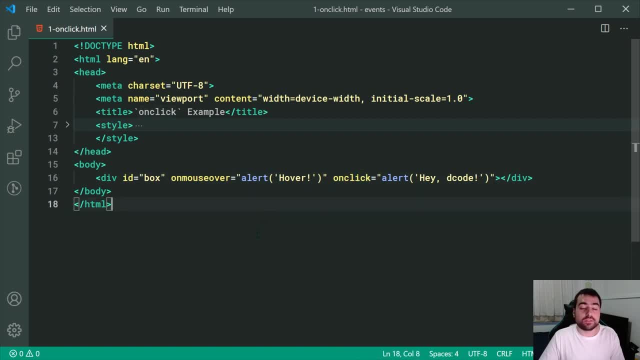 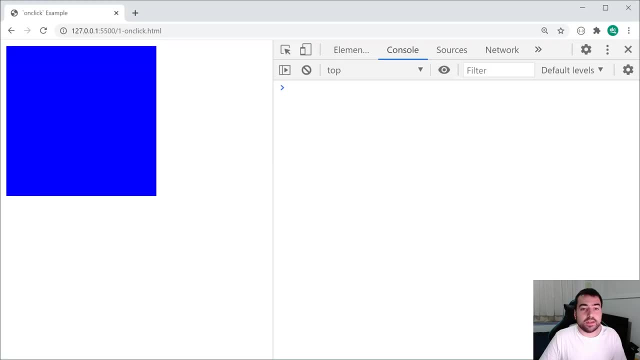 right here The onMouseOver and the onClick And of course that is perfectly fine and valid. So now saving this right here. going inside the browser, we can see: if I was to hover over the actual box, we get hover right there. If I was to then click on the box, we also get. hey, decode. 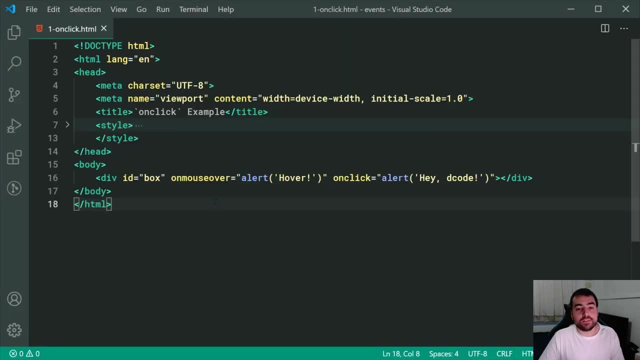 So right there, we can see an example of adding the two events right there. Now, what is the problem with this style of event handler? Well, you can't actually do much inside these quotes, Okay. So of course you can do quite a few things inside here, but of course, once your project. 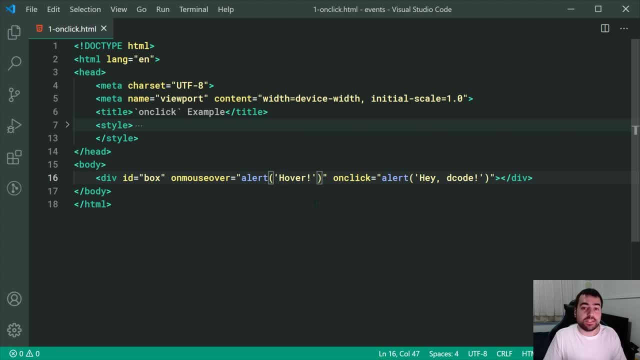 gets more complex and you want to do many different things inside the event handler. you're kind of restricted as to what you can do inside here, and it can get very messy quite quickly, So the better option is going to be to essentially put all of your JavaScript code inside its. 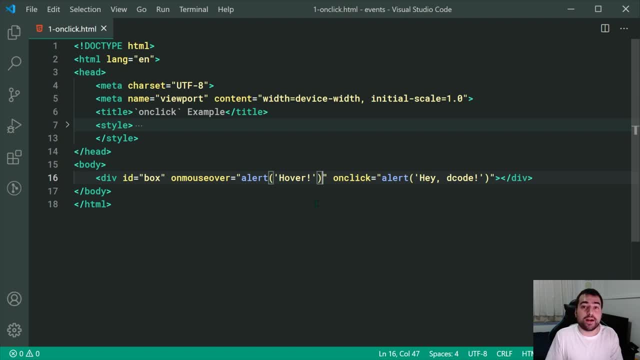 own separate, you know section of the page or its own file and then do your event handling inside there Instead. it makes it much easier to work with And, of course, that brings us to the addEventListener function. Okay, so addEventListener is going to be the preferred way for you to add events to your 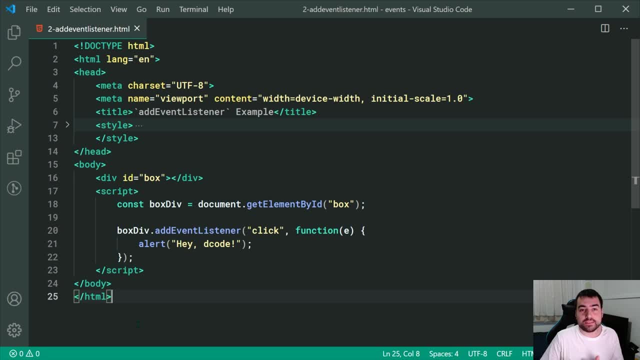 JavaScript code and, of course, your web page. So right here we can see we get a very similar example. I've got the exact same div with an ID of box, But now I've opened up this script tag right here and I've specified some JavaScript code. 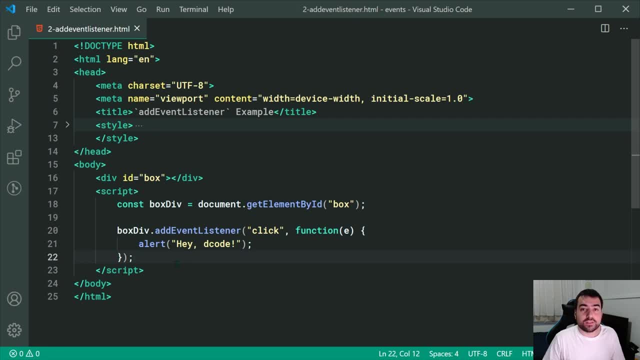 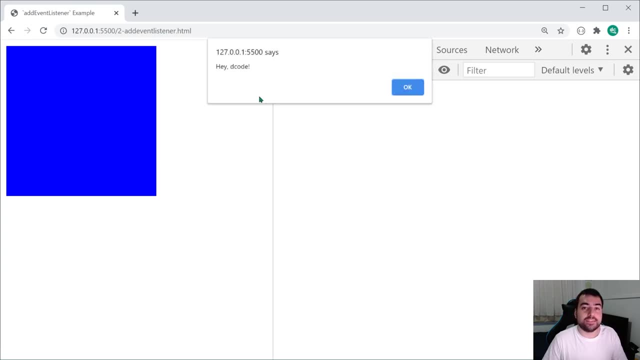 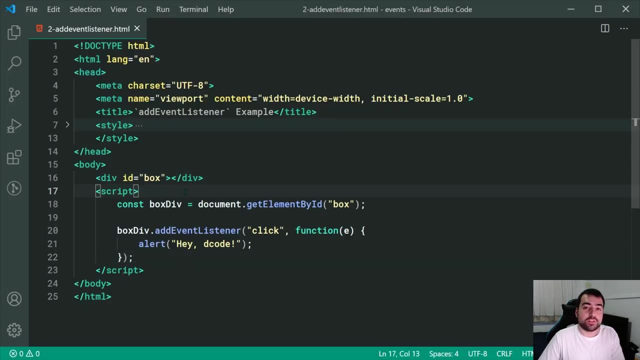 Okay. So essentially it's going to do the exact same thing and I can show you this right now. So, going inside the browser, we can see, upon clicking on the box, we get right here, hey, decode. So now looking at the actual code itself, we can see in the JavaScript the first line of: 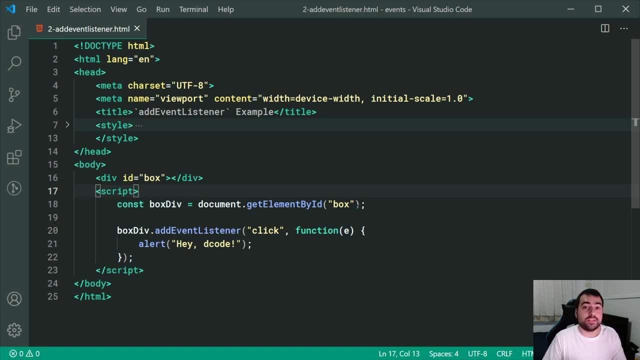 code here is simply grabbing the actual div from the HTML. So right here I'm just saying a new constant or a new variable called box div is equal to documentgetsElementByID And I'm passing in box right here. So for those of you who don't know, essentially if I pass in box right here it's going to. 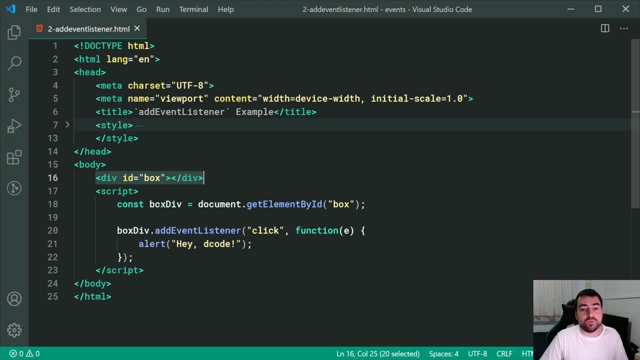 grab this div. and now, essentially, this div refers to this box div right inside the JavaScript code. So now I'm just simply saying box divaddEventListener and I'm passing through here the click event. So similar to the previous example where we had the mouse over. 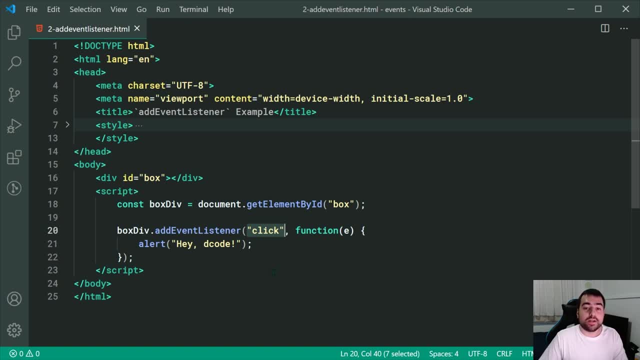 the previous example where we had the mouse over. you can also pass in mouse over inside here and that is also going to work. Like I mentioned earlier, there are many different JavaScript events to use, so you're going to have to do your own searching and find out what you need for each different scenario. But let's go. 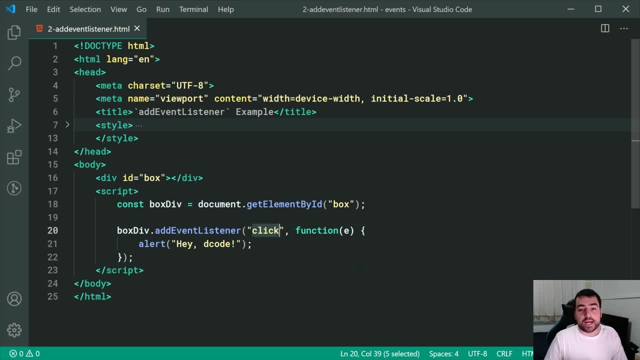 back to the basic click event right here. After this, we're simply specifying a JavaScript function right inside here and I'm accepting the event object right there. So we're going to get to this very shortly, but for now we can simply ignore that and then going inside the actual function body itself. I'm then saying: 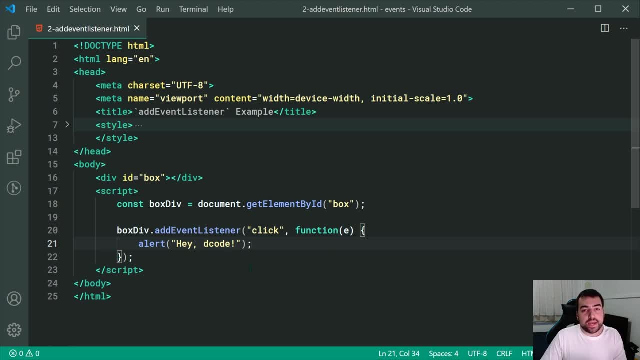 alert, hey, decode. So essentially we're moving the alert call from inside the HTML in the previous example to this function right inside here, and this makes it a lot easier to work with and essentially you're going to have a much better time writing your JavaScript code inside the script tag or an external file, compared to 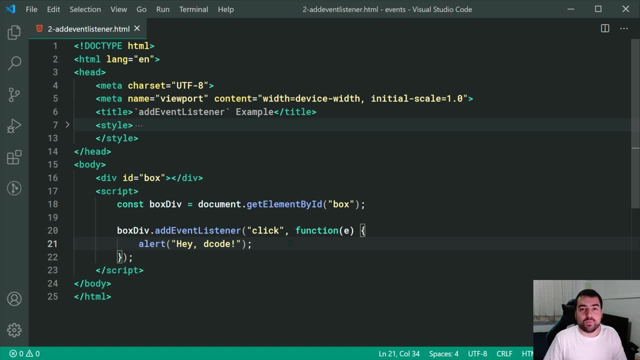 inside the HTML. So of course we saw how that one works. Now what if I was to? instead of specifying the function right here, we can actually specify externally. So this right here is another example of what you might see. So if I was to, 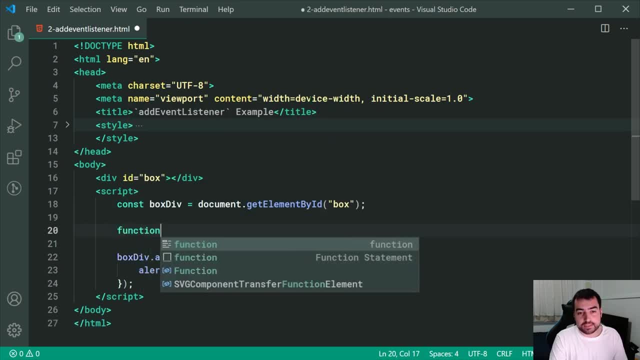 specify a function right inside this function, right here, and then I'm going to go inside here. I can say function and call this function handle box click. So essentially this function is going to do the job of handling the box click. So now I can also accept the event object, as we did earlier, and then I can simply move. 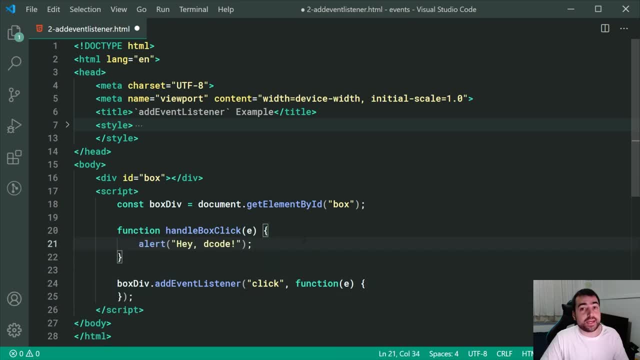 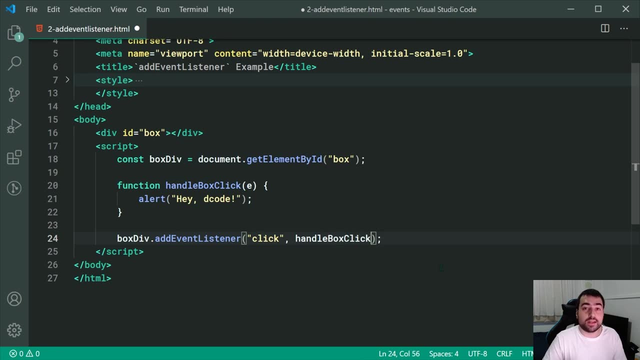 the alert code inside here, and then, instead of having this function right here, I can instead just say: handle, box, click, just like that, And that is a function that is going to give us the exact same result. It is simply just a different way of writing it, and you might see this example or style also. So 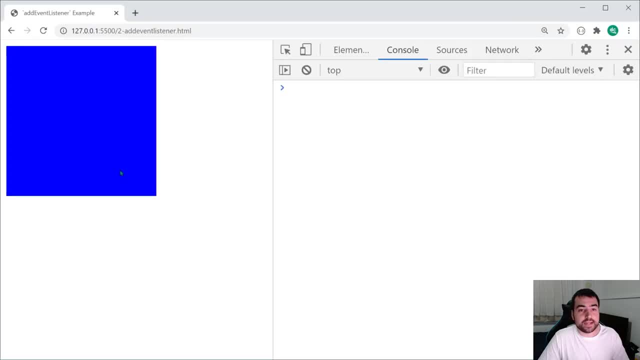 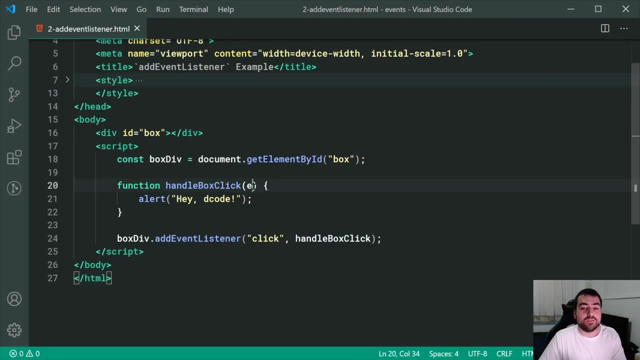 if I was to save this, we can see. we get the exact same result. We can click and we get hey decode. So now we're going to move on to taking a look at the event object right here. So let's look at that right now. 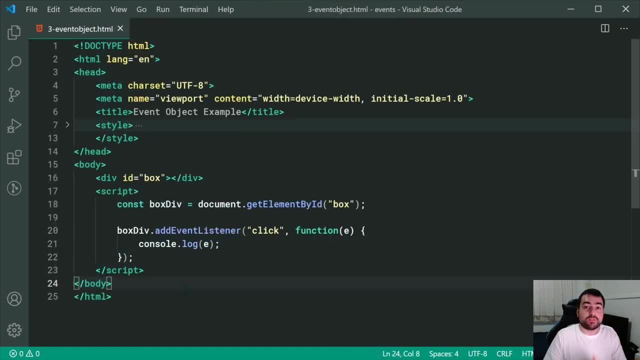 Okay. so, moving on to the event object, I'm referring to this e right here Now, I know this e confused me quite a bit when I first started learning JavaScript, but it's actually very straightforward in what it actually does. So, essentially, this e or the event object contains information about the event which has 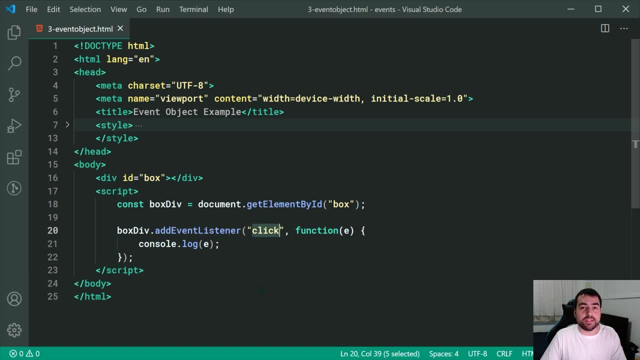 just occurred. In the case of the click event, you can find many different pieces of information about that click. For example, you can see if the user was holding down the alt or the control key when the click occurred, or even the position of the mouse Now to gain access. 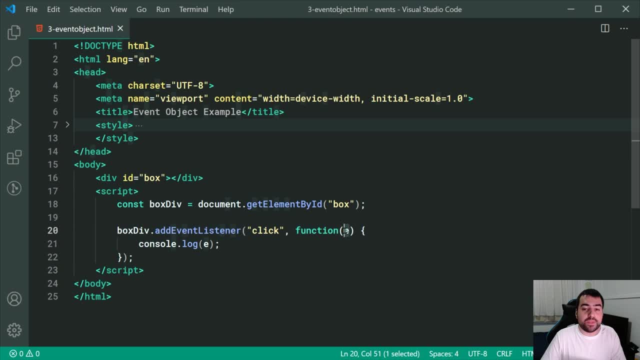 to the event object. you simply pass through a name for the event object right here inside the function. Now, of course, you can call this whatever you want. For example, it doesn't need to be e, We can say ev, or we can even say event. 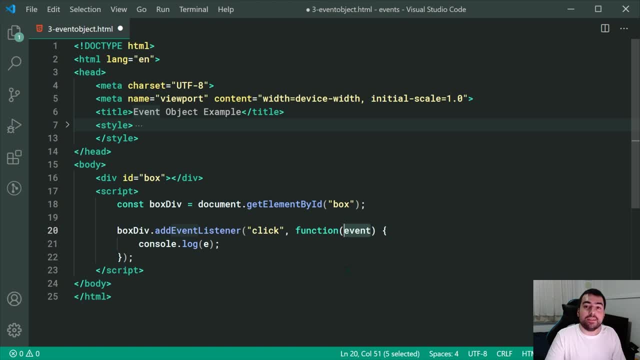 right here. Realistically, we could say absolutely anything like decode, for example, and that is also going to work, but it is a must convention to simply use e or ev as the name for the event object. Okay, so, that being said, we can then reference or use the object inside the function by: 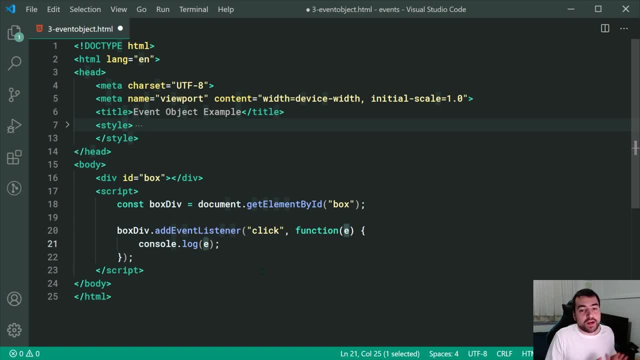 saying e just like this. Now, right here, I'm simply saying consolelog and I'm passing through e. So essentially, this consolelog is going to tell me information about the actual objects right there inside the JavaScript developer. So now, if I was to save this right here and go inside the browser, I can then using 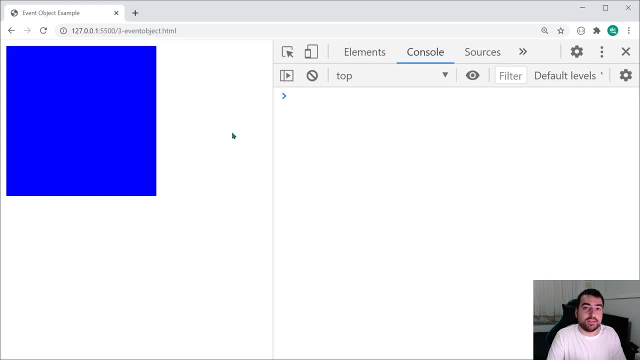 F12, you can toggle the developer tools right inside here and you may need to switch to the console output right up here to gain access to, of course, the console. So now, if I was to click on the object, we can see, so on the div, we can. 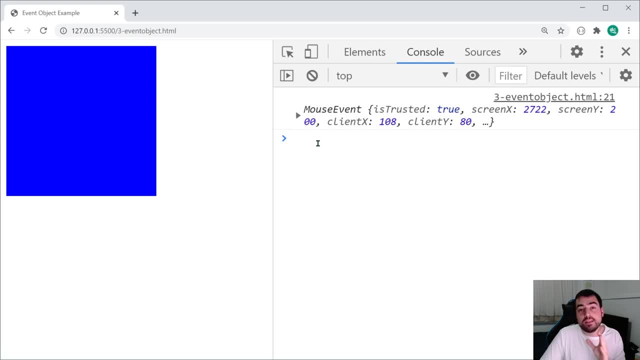 see right here we get the mouse event inside the console right here and notice how it says: mouse event. There are many different event objects in JavaScript because of course this one right here was a click event. A click event relates to the mouse, so of course we get the mouse. 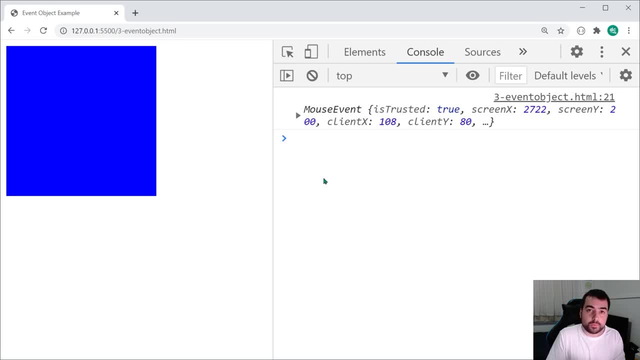 event. There is also the keyboard event, for example. So now, going inside the actual object itself, we can see there are many different properties related to the event which has just occurred. For example, we gain access to the client x and the client y, and these: 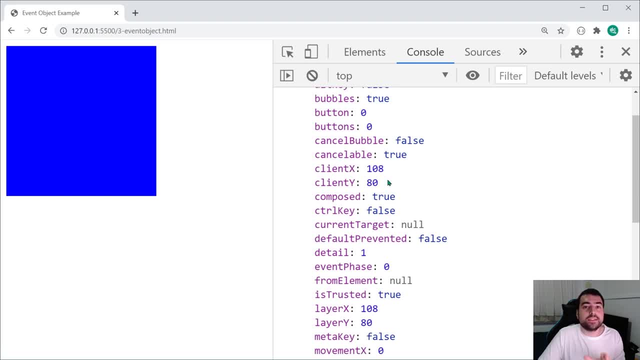 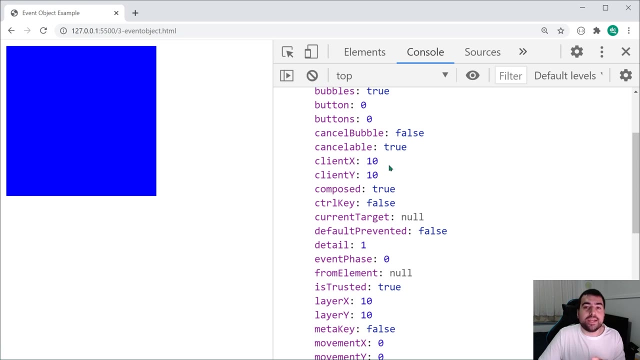 are just the mouse coordinates. when the click occurred, We can see we get 108 and 80 right inside here. If I was to click again this time. in the top left corner we can see the client x and the client y are much lower at 10 and 10.. We also gain. 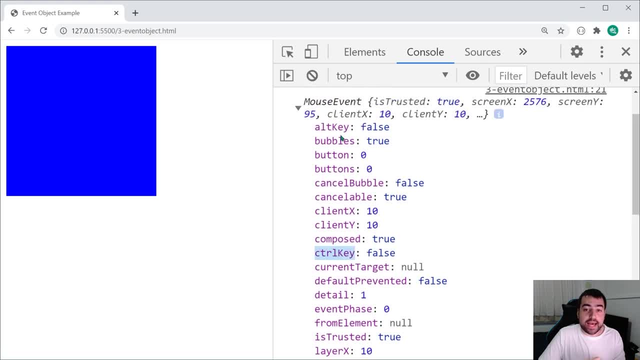 access to things like the control key and the alt key, which of course tell you if the alt or control key were pressed or held down when the click occurred. For example, we can see now the control key is set to false, but if I was to hold the control? 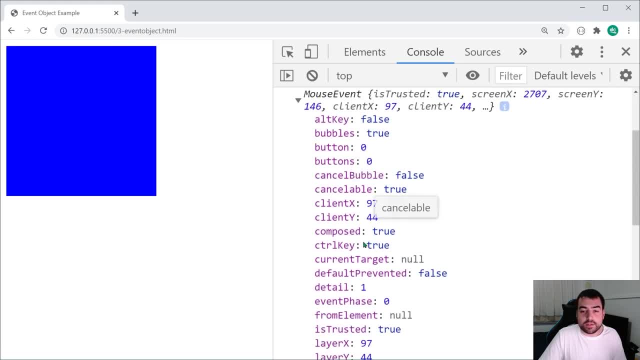 key and click again. we get right inside here. control key set to true. So of course, depending on your own scenario or use case, you're going to find these properties useful. Okay, so of course it's going to depend on your own project, what you're doing. You may not need to use. 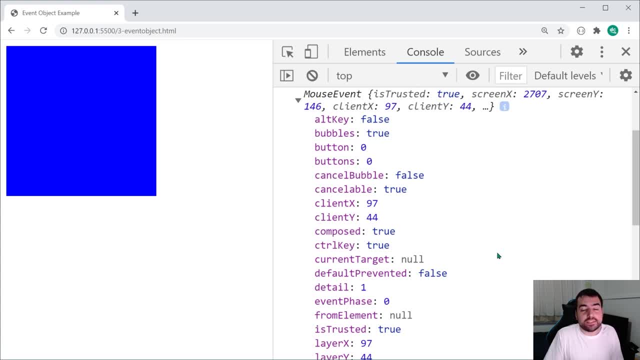 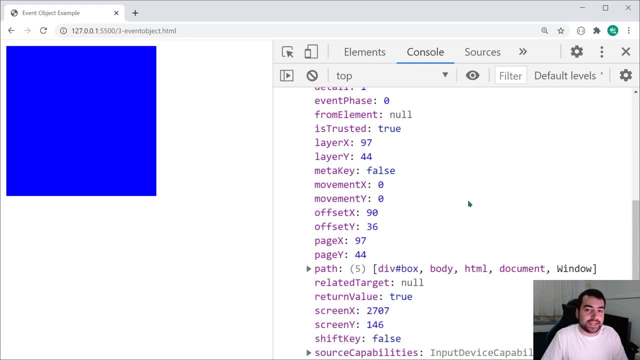 any of these properties, and that's perfectly fine, but in many cases, you may need to go and access to these different information regarding the event to, of course, do different things. Okay, so let's move on now to the usage of the arrow functions in comparison to the. 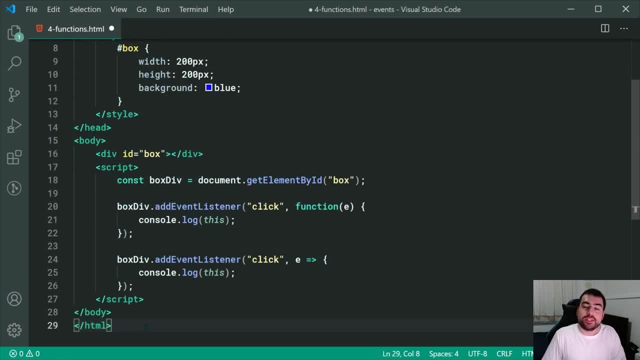 standard JavaScript functions. Okay so, moving on to the final part of today's video, and that is going to be the difference between standard versus arrow functions when it comes to your event handlers. Okay, so, right here we can see. I have two examples of the usage. 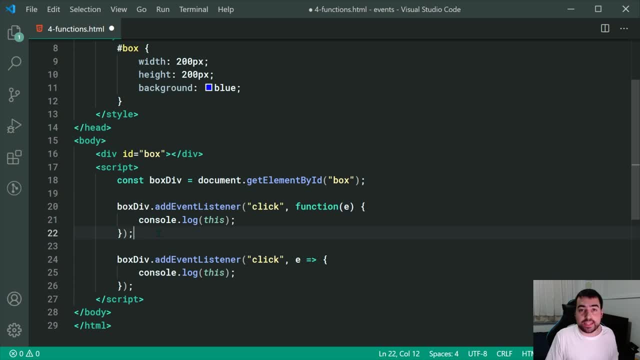 of the addEventListener method. Okay, so right here we can see the first example is very similar, if not the same. in fact, it is the same as our previous examples. We're simply saying function and then, of course, taking through the event object, and then we're simply: